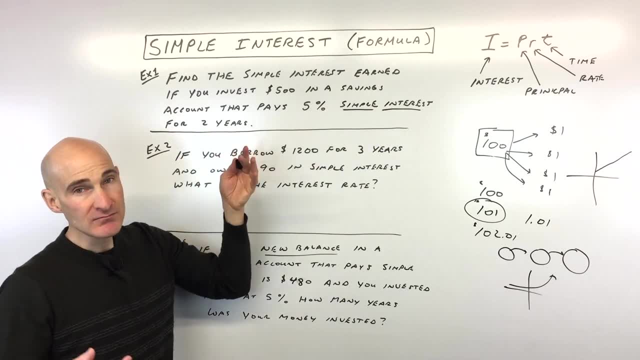 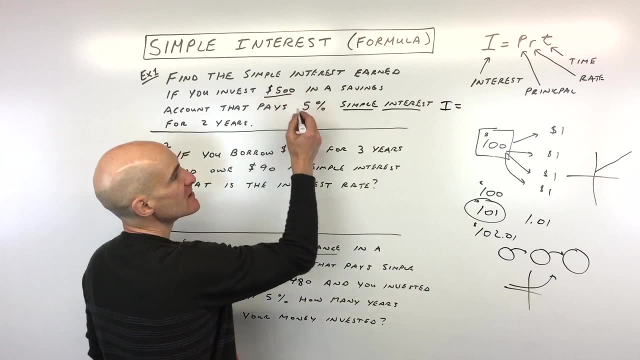 But let's just say simple interest for two years. Okay, so then what we're going to do is we're just going to substitute in these values. So we've got. I is what we're trying to calculate. P is our principal, which is the $500. 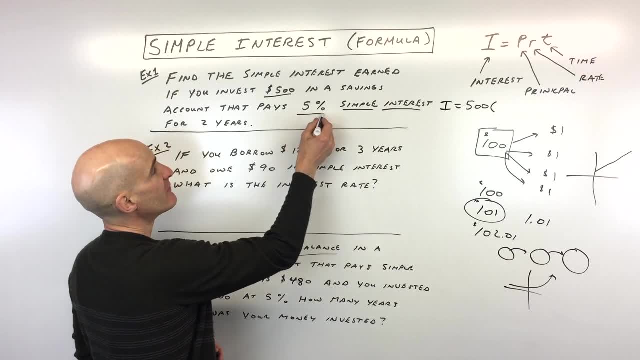 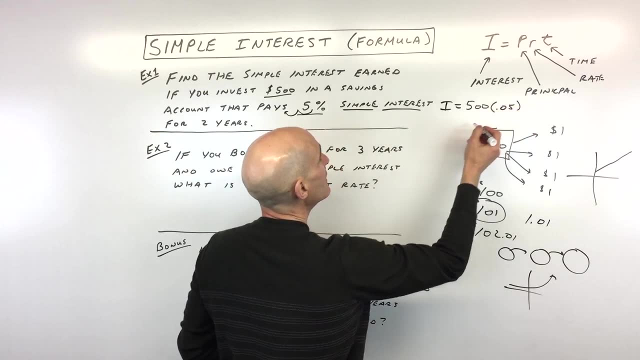 The initial amount, The rate, which is 5%, But we want to convert this to a decimal, So we have to move that two places to the left, So that's going to be .05.. And then the T, the time, that's two years. 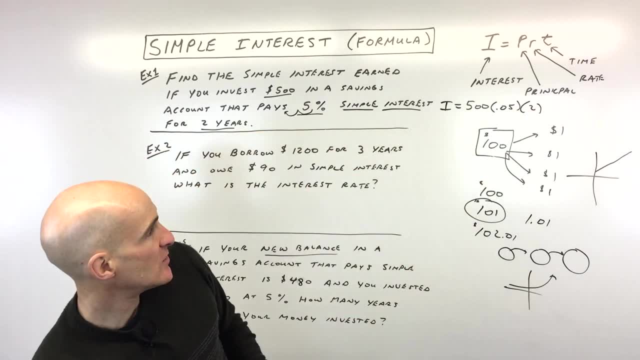 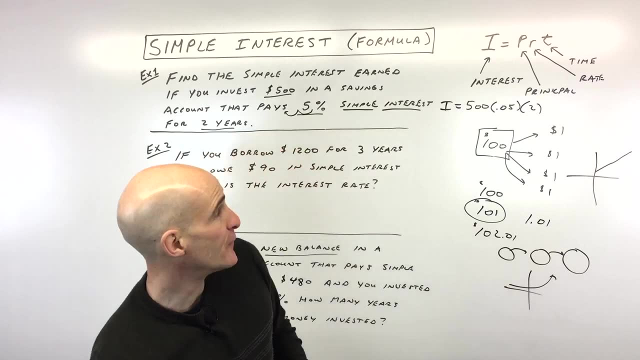 So we're going to multiply this by two. So let's go to the calculator. Let's see what that comes out to. Let's see We've got 500 times .05. times two years, That comes out to $50.. 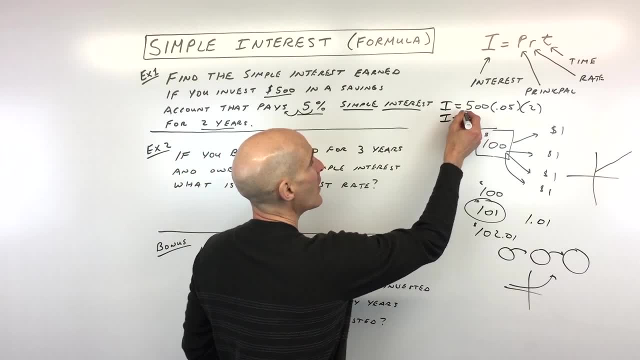 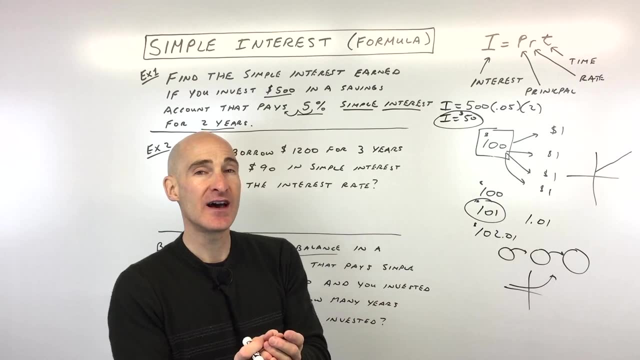 Now if the question asks you: you know how much money do you have After two years? Well, you'd have the $50 plus the initial amount, the $500.. You'd have to add those together: $550.. So that's our first example. 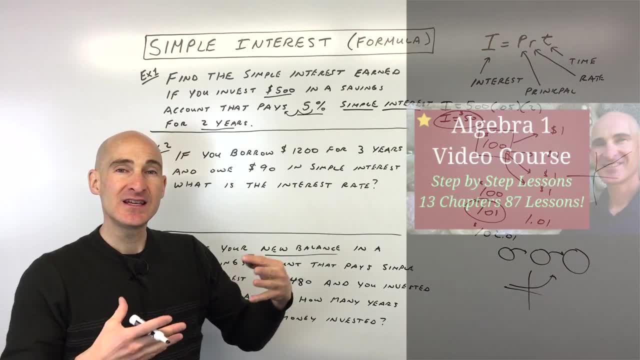 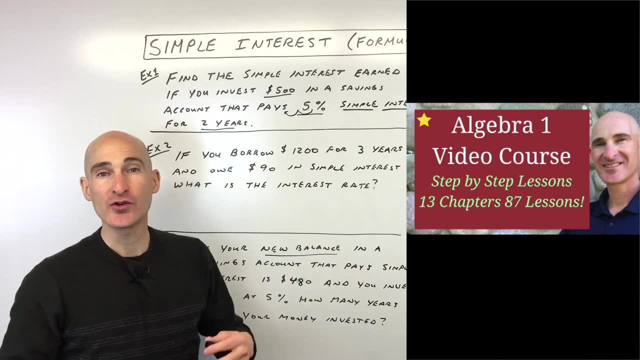 Let's go into our second example, But before I do that, if you're getting into Algebra 1 or you're in Algebra 1 already and you want additional help, check out my Learn Algebra 1 video course for sale. It goes through 87 video topics, taking you step by step by step through the beginning of Algebra 1,. 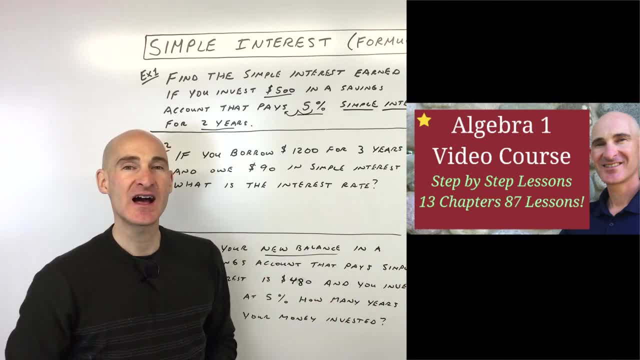 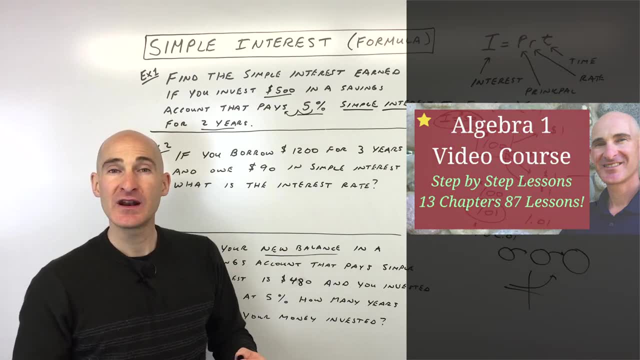 through the middle all the way to the end, building on the previous concepts. You can check out the 13 free lessons to see if it's a good fit for you, But it's been taken by a lot of students already. They've benefited. 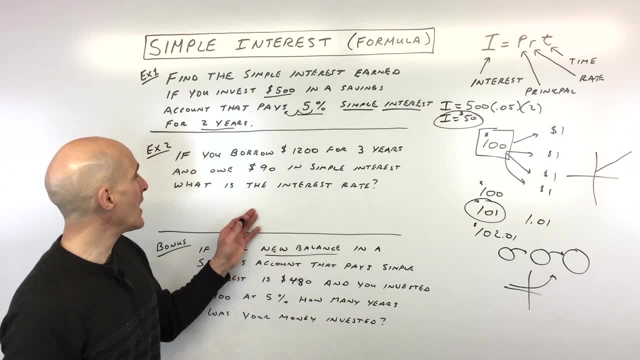 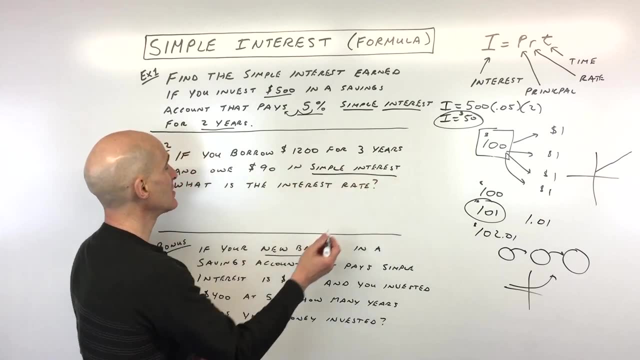 I know you will too, So go ahead and check that out. But let's go to example number two now. It says: if you borrow $1,200 for three years and you owe $90 in simple interest, what is the interest rate? 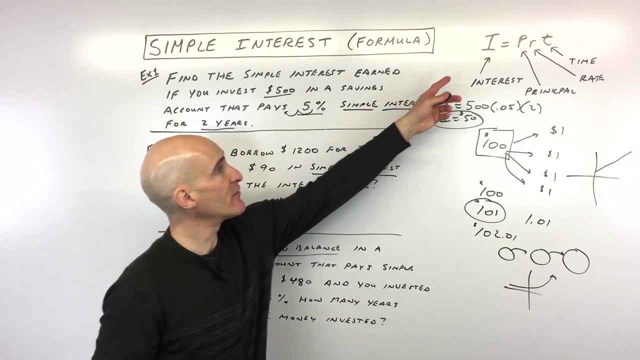 Okay. so this problem is a little bit different, in the sense that we're not actually solving for I, We're solving for R. Okay, so the first thing that I like to do and I recommend to you know, the students that I tutor- 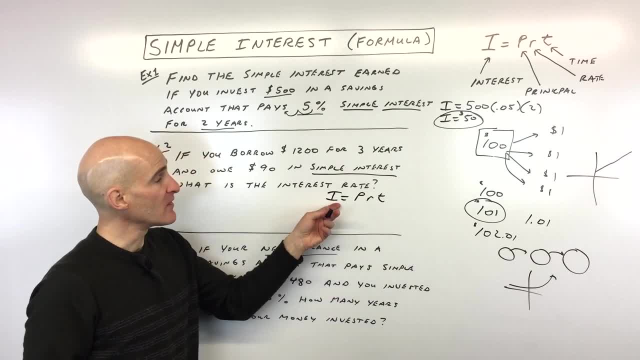 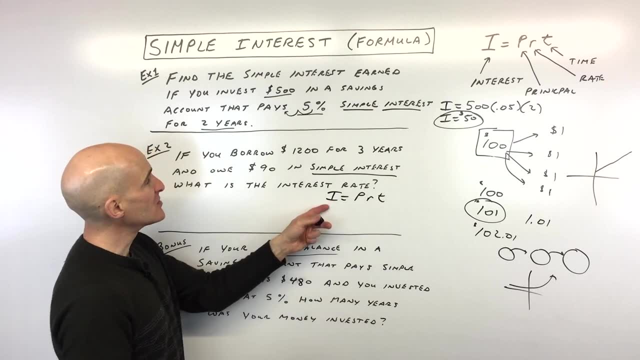 in person is go ahead and write down that formula you know. first, Number one, it helps you to memorize it. But number two, it kind of helps you to organize what you know and what you need to solve for. So in this case we know that the interest is $90, right? 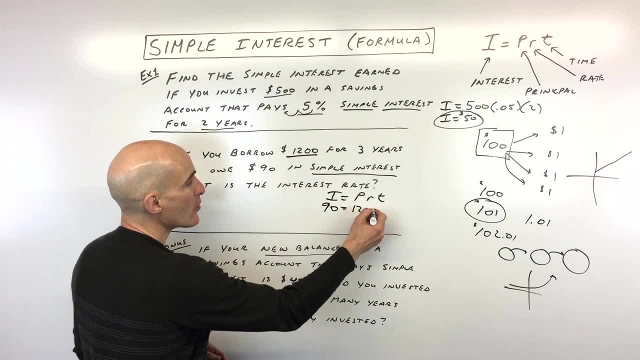 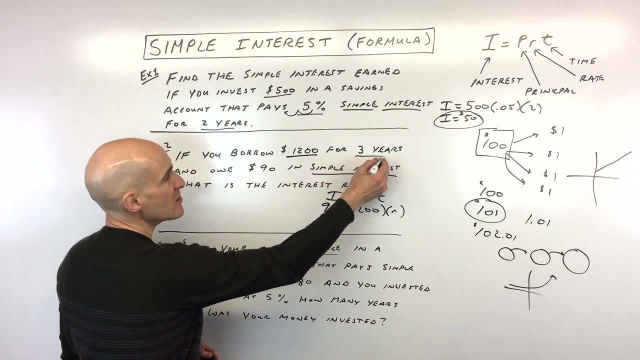 And the principal. we know that's the starting amount. That's the amount that you're borrowing, the $1,200.. The interest rate, we don't know. So let's just call that R And then the T. the time is three years. 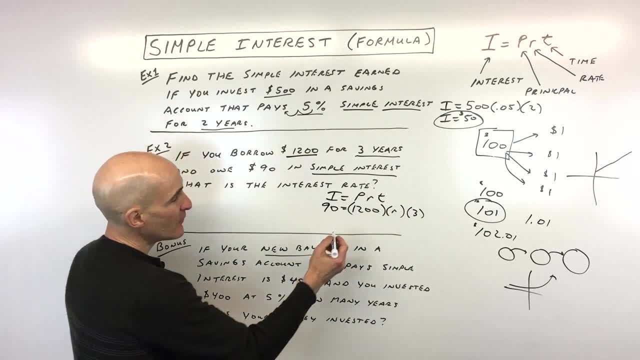 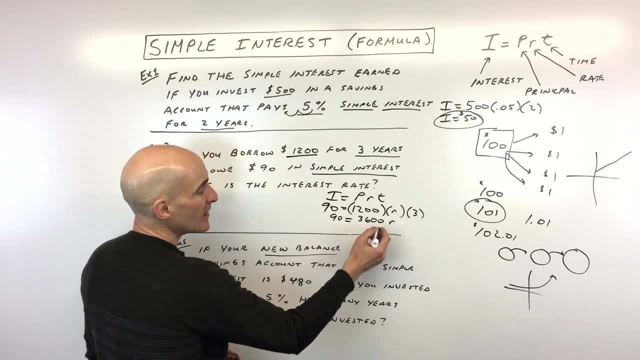 So we're going to put in three in place of T. So if we simplify here, $1,200 times three, It's 3,600 times R, equals 90.. We just want to get R by itself, So we're going to do the opposite of multiplying by 3,600.